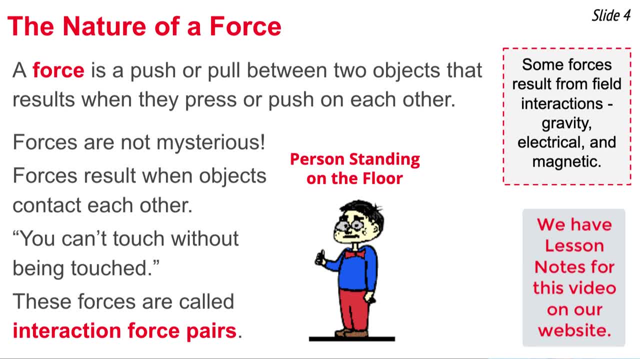 there's contact between the feet of the person and the floor. That contact results in an interaction force pair. We would describe it like this: The person pushes down on the floor and the floor pushes up on the person. These two forces act on different objects in opposite directions. 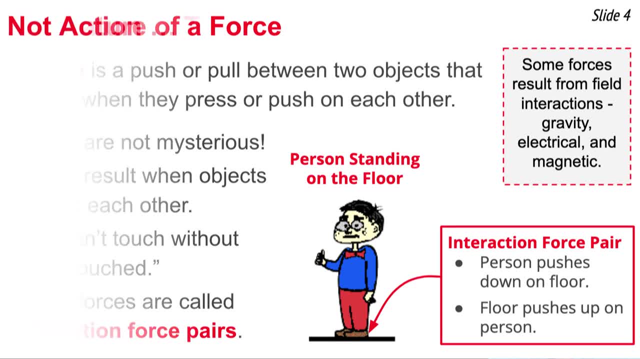 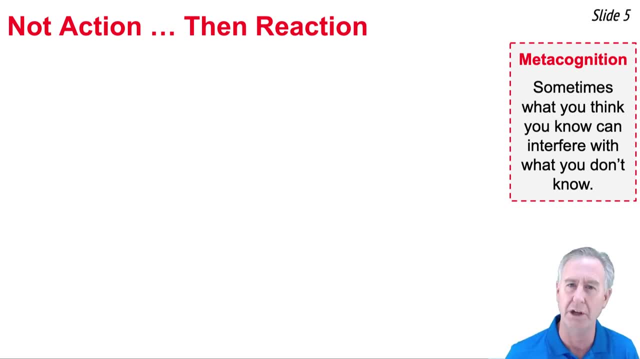 and are of equal strength. That's Newton's Third Law. You know, it's often the case in physics that the things that we think we know interfere with the things that we don't know, And that may be the case when it comes to the. 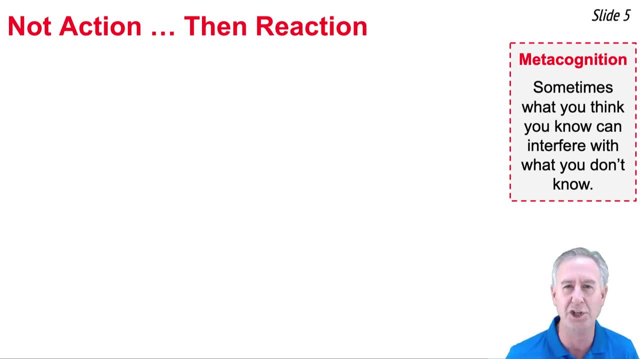 Third Law of Motion, because we often call this the Law of Action, Reaction, And it gives you the idea that there's some sort of action taking place and then the reaction force is the result or consequence of that action. But that's not what the Third Law means. 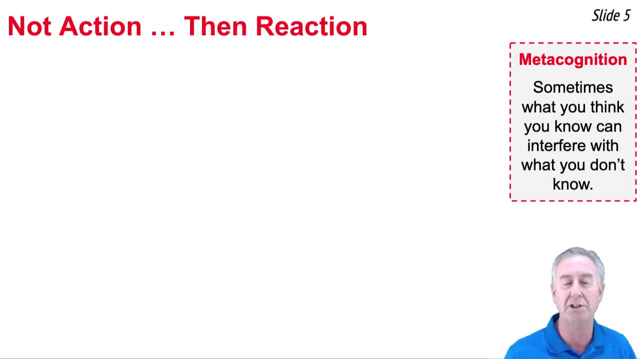 It's not like I push on a book and the result of that is the book's arm pushes back on me. That's not how it works. The idea is that when two objects contact each other, there's this contact interaction that results in a pair of forces. 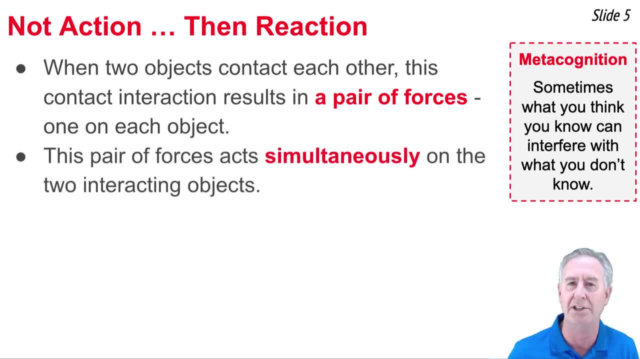 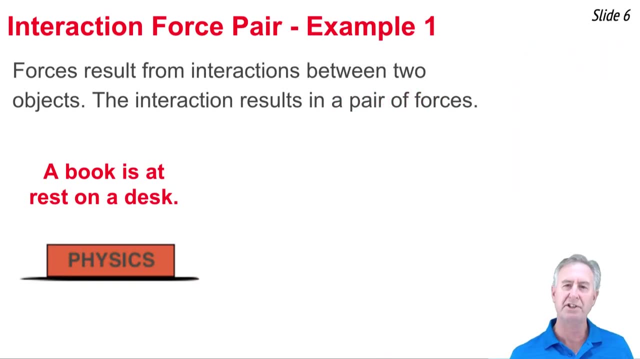 that act simultaneously on each of the objects. It really isn't like the idea of action then. that's not how it works. It would be better if we called this the Law of Interaction. Force Pairs, That would be the better way to think of it. So Newton's Third Law suggests that forces result. 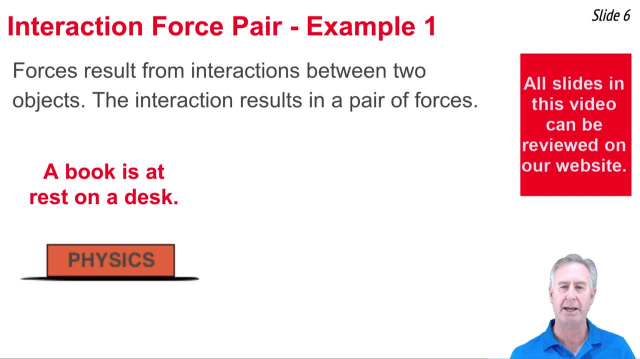 from interactions between objects. Let's look at a couple of examples. Let's consider here a book that's at rest on the table. The book touches the table and since you can't touch without being touched, the table touches the book. That's an interaction that results in a pair of forces. 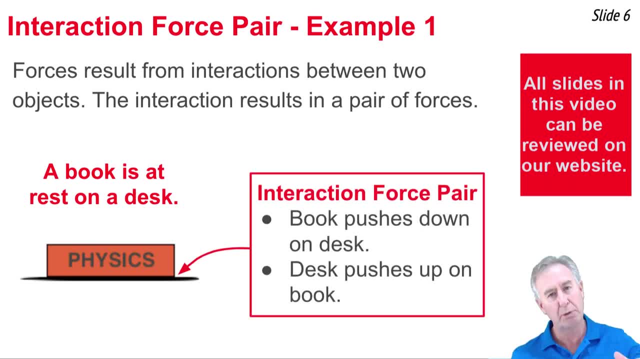 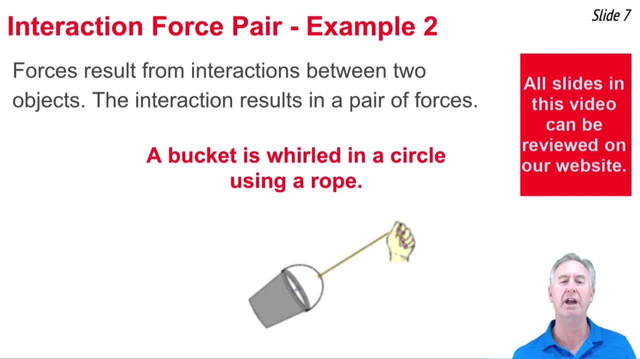 Here's how we would describe that interaction: The book pushes down on the table and the table pushes up on the book. Let's look at a second example. Here we consider a bucket being rolled in a circle using a rope. The rope touches the bucket and since you can't touch without being touched, the bucket, 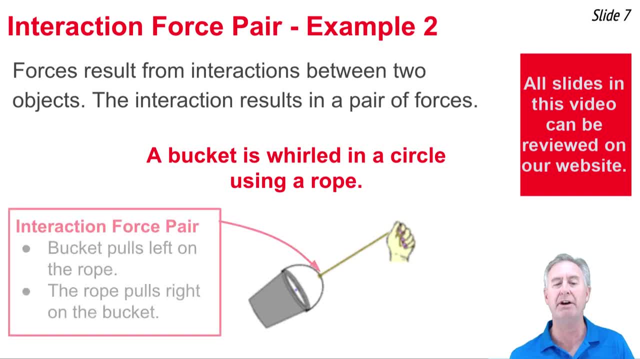 touches the rope, And so here's how we would describe that interaction force pair: The bucket pulls leftward and downward up on the rope, and the rope pulls upward and rightward up on the bucket. This is what Newton's Third Law suggests: that forces result from interactions and that 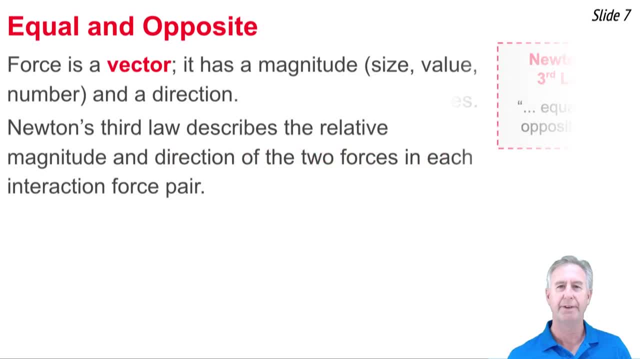 interaction results in a pair of forces. So Newton's Third Law describes these individual forces and the interactive force pairs as being equal and opposite. Here's what we mean. Force is a vector, that is, it has a magnitude, a numerical value, and it has a direction. What newton's third law does is it describes both the magnitude and the direction. 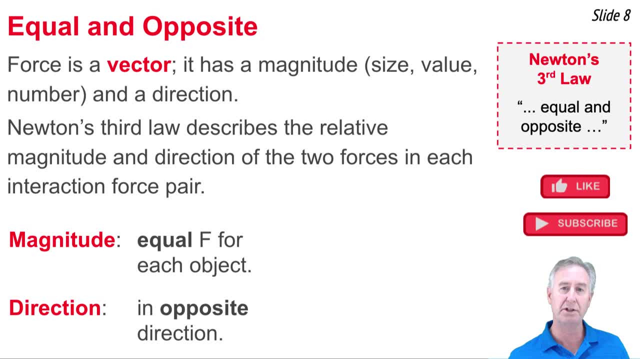 two individual forces. As for the magnitude, it describes it as being equal on both of the objects. and as for the direction, they will be in the opposite direction on the two objects. Here's an example: Let's suppose a ball is moving to the right and it contacts a catcher mitt as shown. Upon contact, there's an. 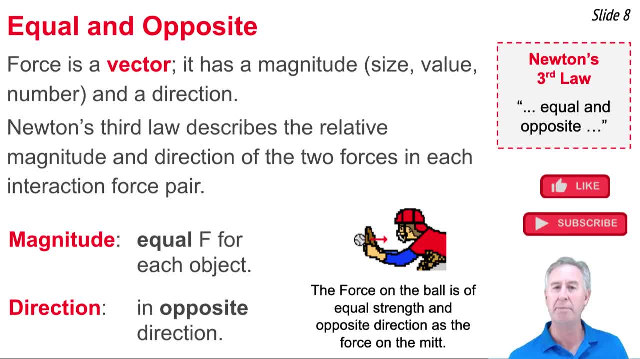 interaction force pair. The ball is moving to the right and so the mitt pushes to the left on the ball and the ball pushes to the right on the mitt. If the force on the ball is 30 newtons, then the force on the mitt is 30. 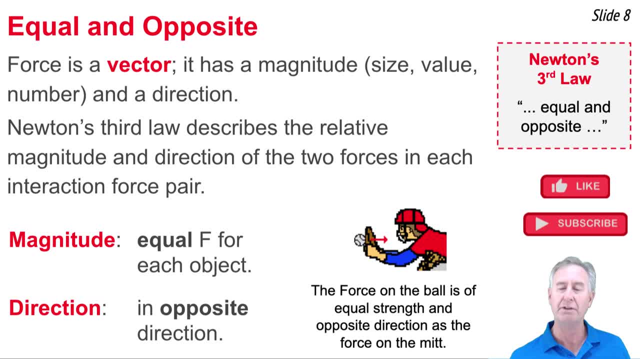 newtons Equal magnitude forces, and these forces are in opposite direction. So the force on the ball would be to the left, the force on the mitt would be to the right. That's what we mean by equal and opposite. Now here's a classic question. 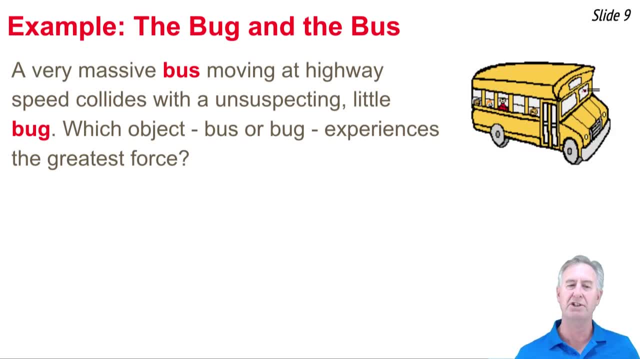 known as the Bug in the Bus question. A very massive bus is moving at highway speeds and collides with an unsuspecting little bug. The question is: upon which opposite direction is this bug moving? The question is: the bus or the bug? is the force the greatest? Your options are? the force is. 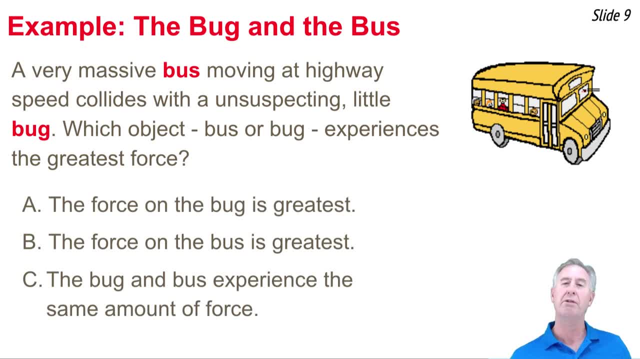 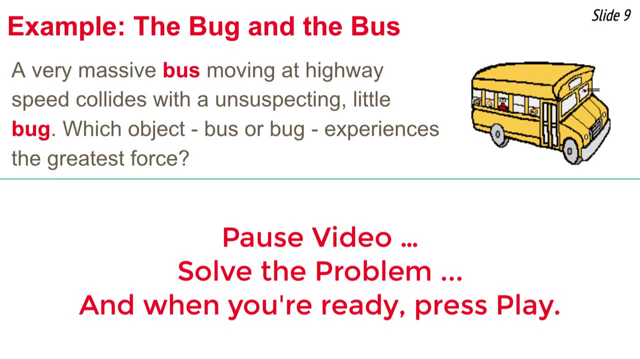 bigger on the bug? the force is bigger on the bus, or the bug and the bus experience the same amount of force. So why don't you pause the video, give it some thought and we'll discuss the answer. The answer is C, According to. 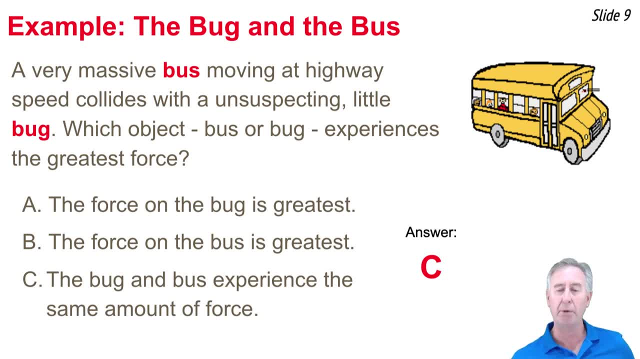 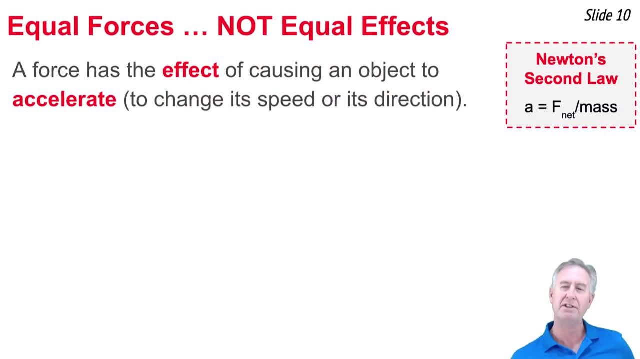 Newton's third law, the forces are of equal magnitude on both of the interacting forces. Now people have difficulties with this and I believe that the difficulty is that they confuse the force with the effect of the force. So Newton's third law states that the forces are equal, but Newton's second 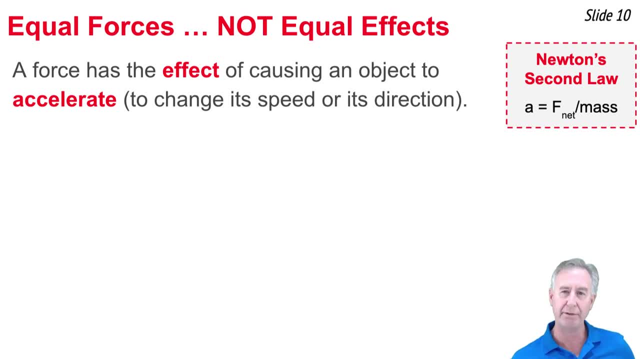 law states that the acceleration that's caused by the force depends both upon the force and upon the mass. So forces, when unbalanced, have the effect of causing an acceleration, and that acceleration depends on more than just the force, it depends upon the mass. So if we apply that to this situation, we'd have to say the force on the bug. 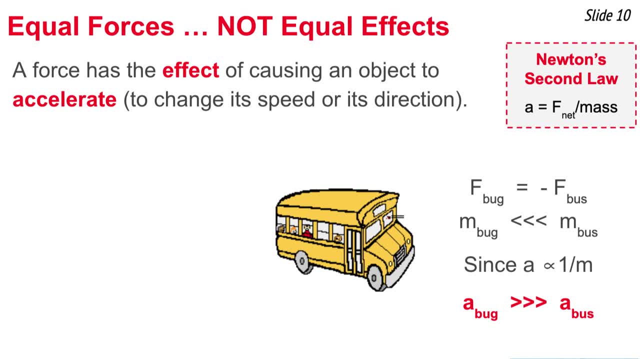 equals the force on the bus. just the opposite direction. but the mass of the bug is much, much less than the mass of the bus And since accelerations depend inversely upon mass, we'd have to say the acceleration is much greater for the. 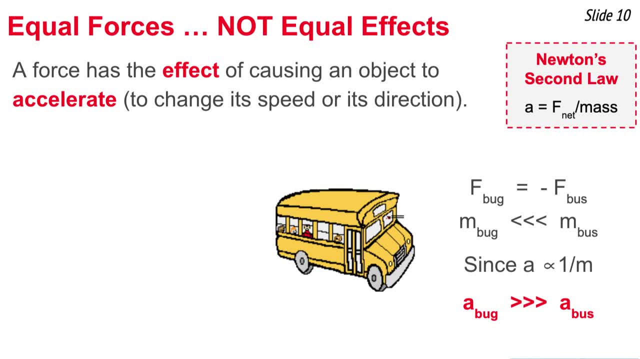 least massive object. The acceleration of the bug is much, much, much greater than the acceleration of the bus. So while the forces on the individual objects are of equal magnitude, according to Newton's second law, the accelerations depend upon mass and are not necessarily equal on both of the objects. 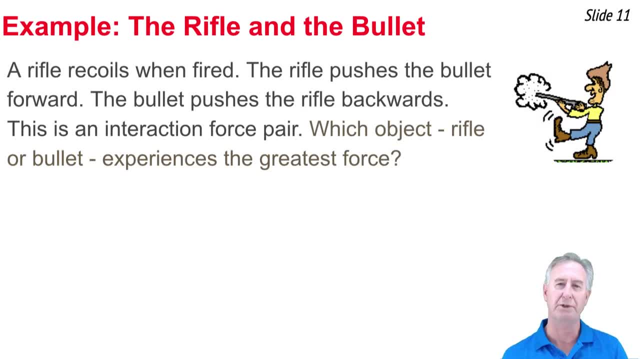 Here's another classic question. A rifle recoils when it's fired. You see, the rifle pushes the bullet forward down the barrel of the rifle and the bullet pushes the rifle backwards. This is an interaction force pair. The question again is which object, the rifle or the bullet? 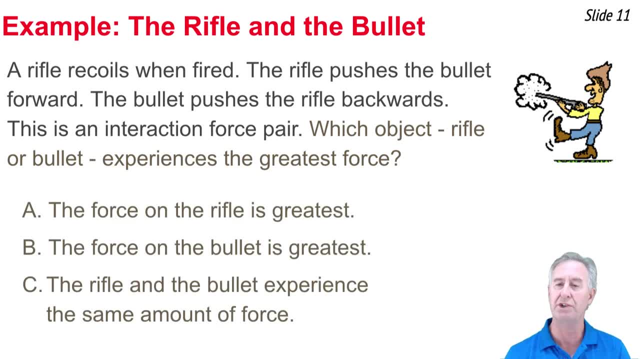 experiences the greatest force, And your choices are: the force on the rifle is greatest, the force on the, the force on the bullet is greatest, or the rifle and the bullet experience the same amount of force. So why don't you pause this video? 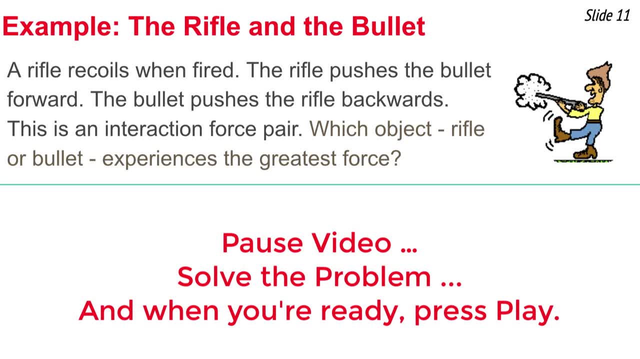 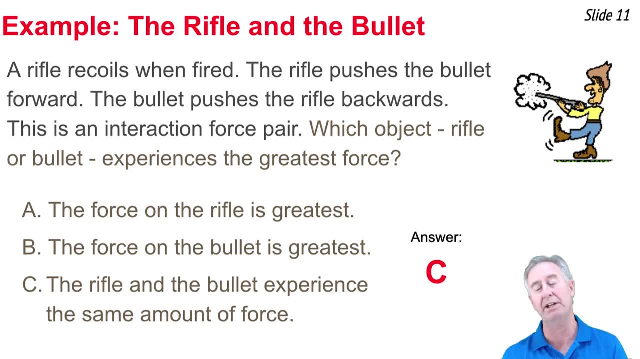 give it some thought and when you're ready, press play. Let's talk about the answer. So the answer once more is C. The force on the bullet is equal in magnitude to the force on the rifle. Now, before you again, you start doing that. 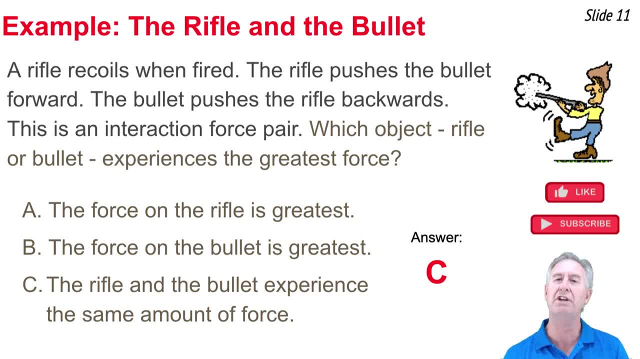 how can that be? Make sure you're not confusing the effect of the force with the force itself. The forces are equal, but the accelerations, the effect of the force, depend upon mass and inversely upon mass, So the bullet having the much.